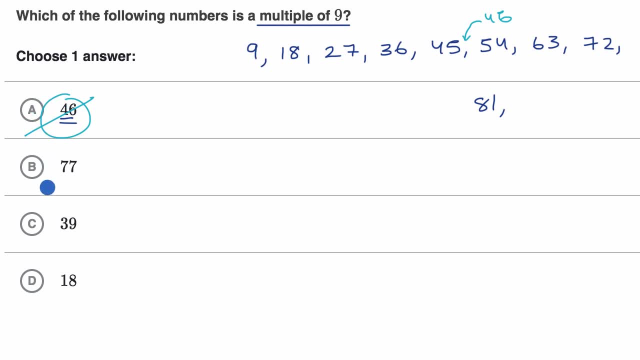 So I am just going to, I'm going to take that one out of the contention. 77 is right over here. it's between 72 and 81.. Once again, it's between two multiples, but not a multiple. 39 is between 36 and 45,, so not a multiple. 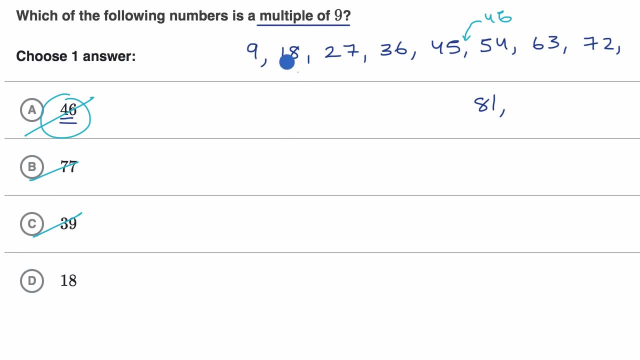 between two multiples. rule that out And we can see very clearly that 18 is a multiple. If I was doing this on my own, I would just maybe be skip counting. in my head I'd be going nine. all right, I don't see a nine, 18,. 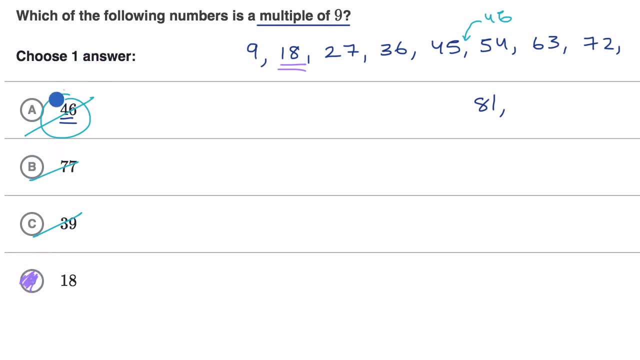 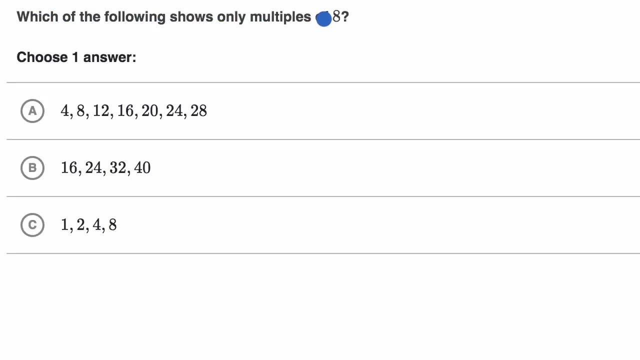 oh, I see an 18,. there you go. especially if I'm only going to pick one choice, Let's do another example Which of the following shows only multiples of eight. So pause this video and think about that. All right, well, I could do it choice by choice here. 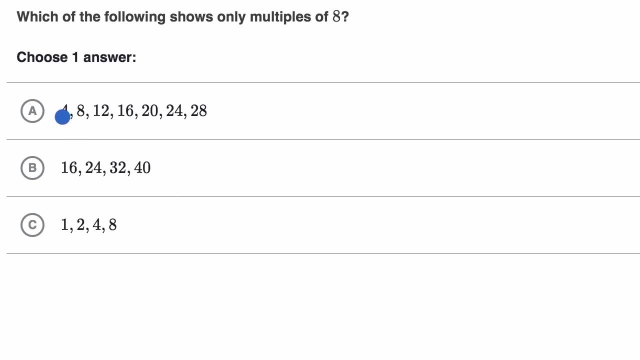 So let's see this. first one is four a multiple of eight. Well, four can divide into eight. We could say that eight is a multiple of four, but four is not a multiple of eight. What whole number am I going to multiply eight by? 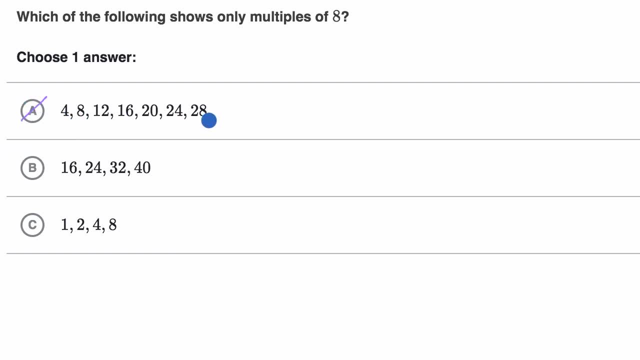 to get to four. So we can rule this out And you can think about what they're showing here. These are actually multiples of four, not multiples of eight. We can skip count here Four eight: 12,, 16,, 20,, 24,, 28,. 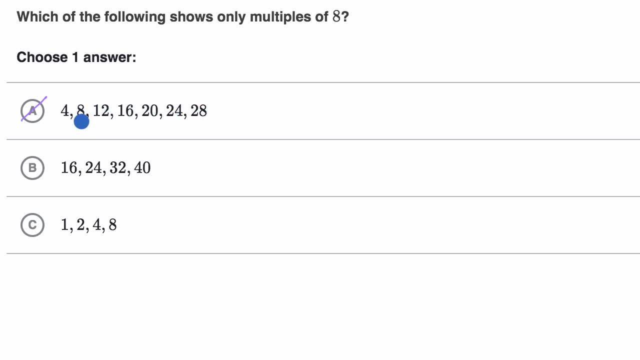 these are multiples of four, not multiples of eight. Some of the multiples of four are also multiples of eight. Eight is a multiple of eight, 16 is a multiple of eight, 24 is a multiple of eight. but not all of the multiples of four are multiples of eight. 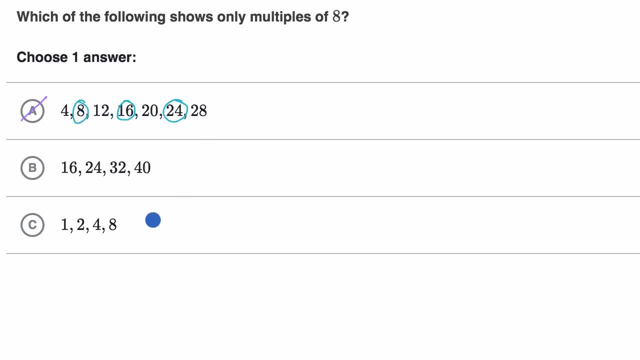 And I think you might be seeing a little pattern here, of which ones are multiples of eight. Now, what about this choice right over here? 16 is eight times two, 24 is eight times three, 32 is eight times four, 40 is eight times five. 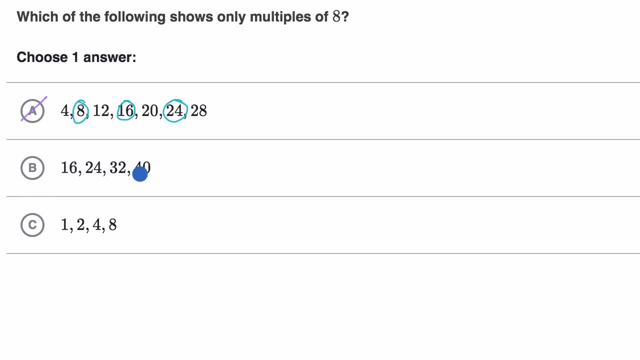 In fact we could skip count Eight, then 16,, 24,, 32,, 40,, then 48,, 56,, so on and so forth, But these are all multiples of eight, so I like this choice. And then over here one, two, four and eight. 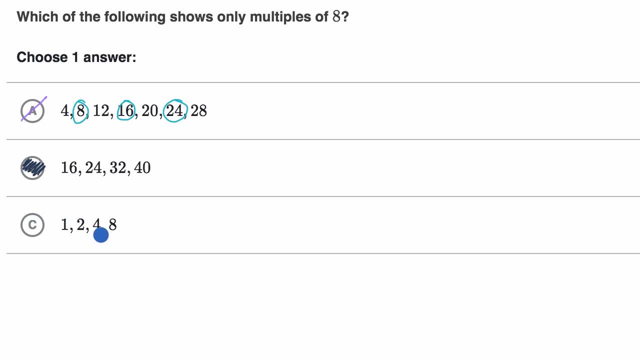 Well, these are showing numbers that can be divided into eight without a remainder. You could think of them as factors of eight. You could say: hey, I could multiply one times eight to get eight. I could multiply two times four to get eight.